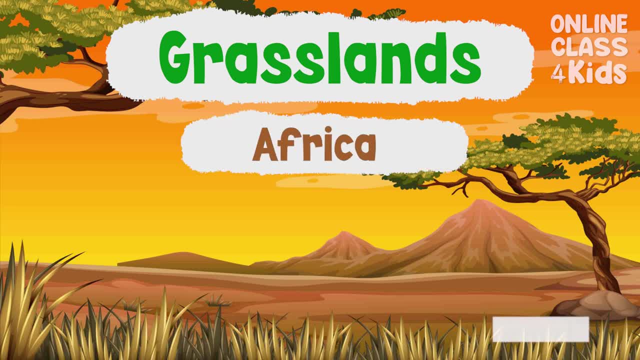 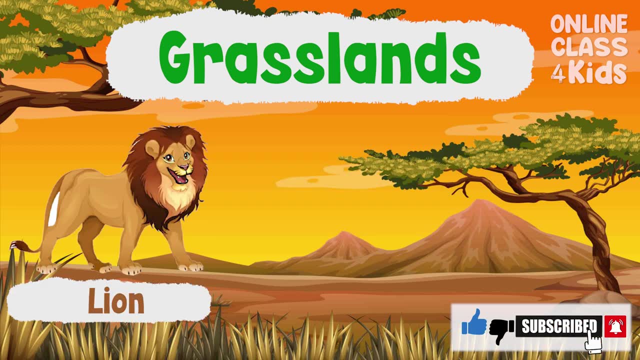 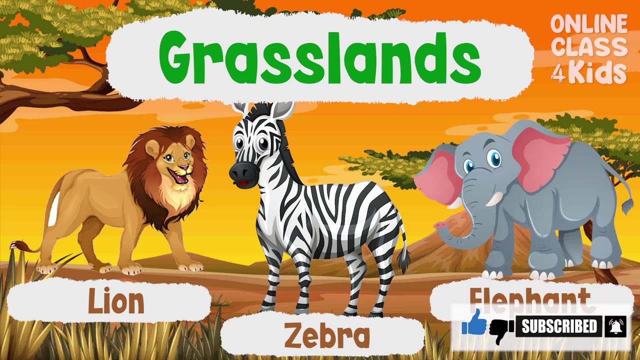 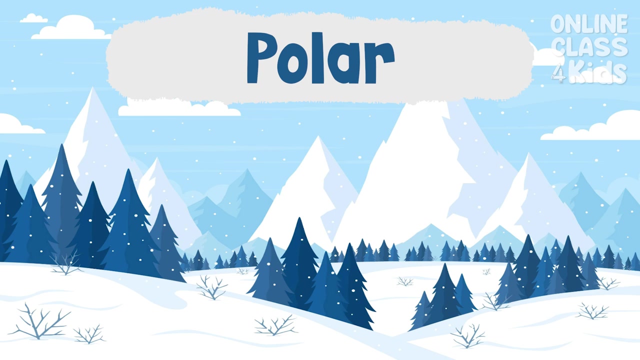 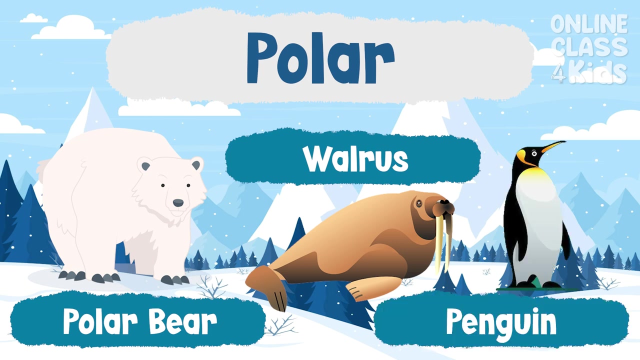 Grassland can be found in Africa, North America and North America. Lions, Zebras and Elephants live in grasslands. Polar habitats are covered in ice and are extremely cold. North and South Poles are polar habitats. Polar bears, walruses and penguins live in polar habitats. 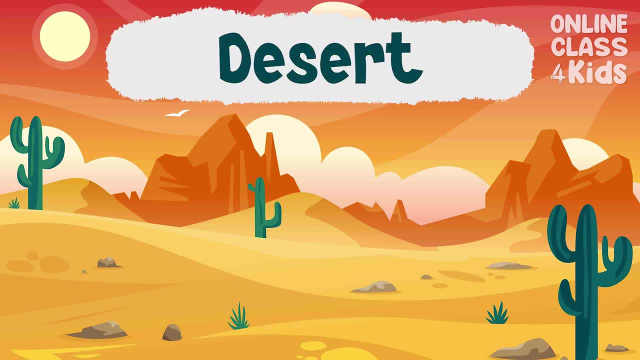 Desert habitats are very hot and dry and don't have a lot of water. Animals living in desert habitats can survive without water for long periods of time. Famous deserts can be found in Africa, North America and Australia: Kangaroos, camels. 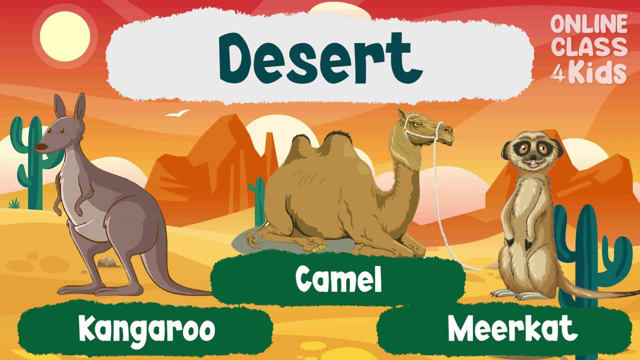 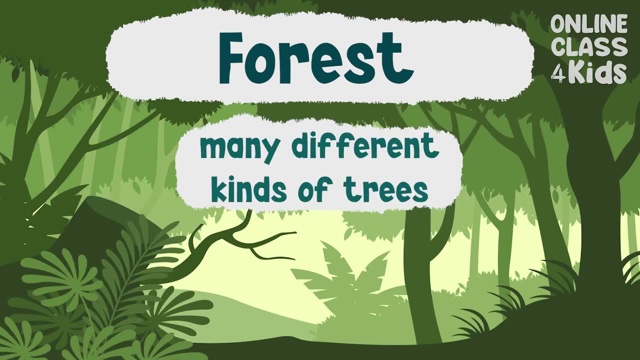 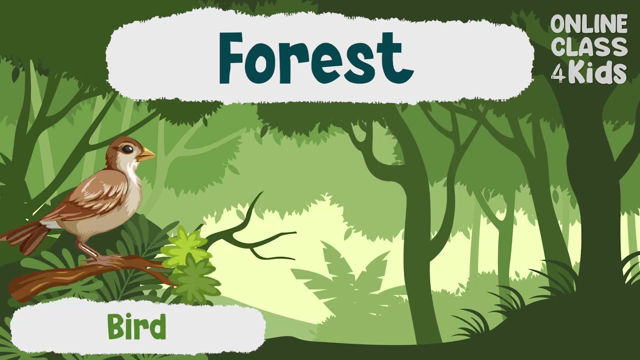 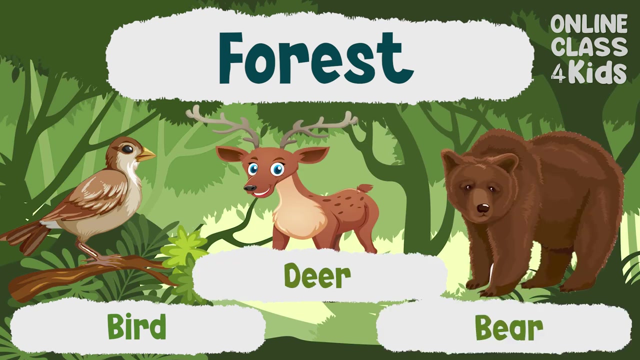 and meerkats live in deserts. Forest habitats are places with many different kinds of trees, Whether it's within the tree roots or trunks, or high up in the branches. forests provide shelter to different animals. Birds, deers and bears live in the forest. 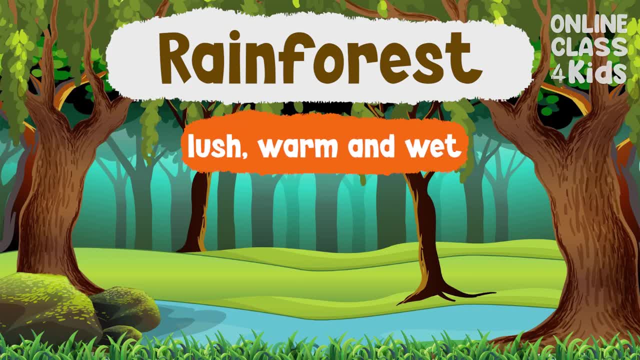 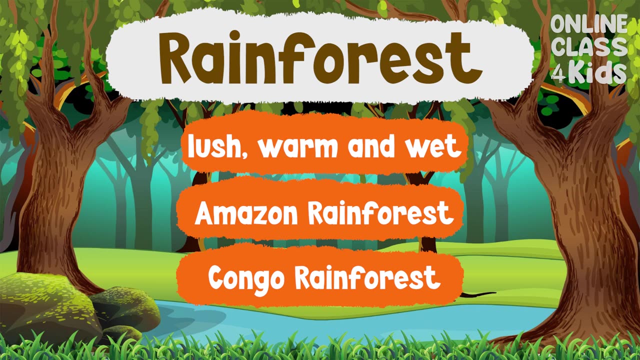 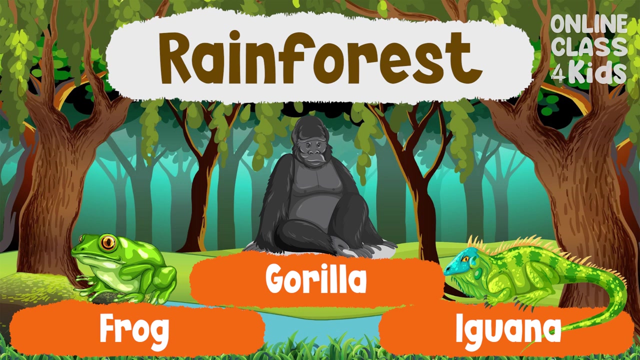 Rainforest habitats are lush, warm, wet habitats. The Amazon rainforest is the largest rainforest in the world. The next biggest rainforest is the Congo. in Africa, Frogs, gorillas and iguanas live in the rainforest. 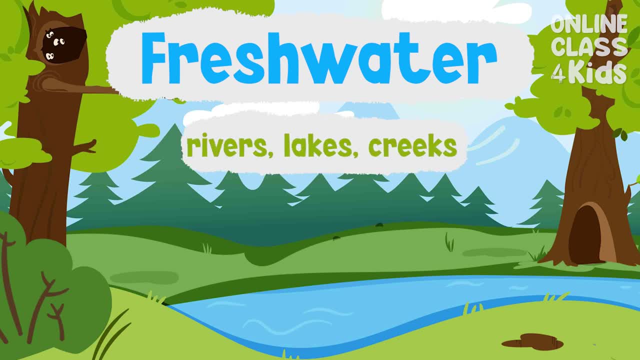 Freshwater habitats include rivers, lakes, creeks, streams and ponds, So are wetlands like swamps and marshes. Freshwater habitats can be found in a lot of countries Like Brazil and the United States: Alligators, ducks. 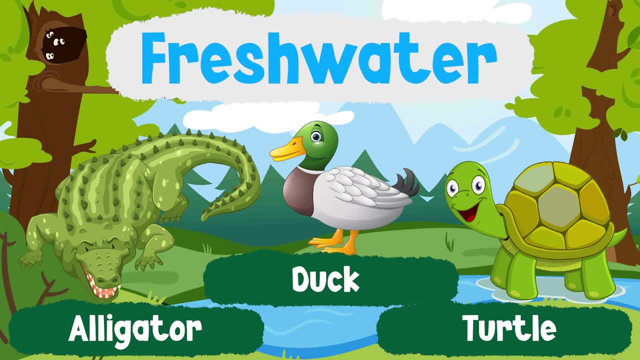 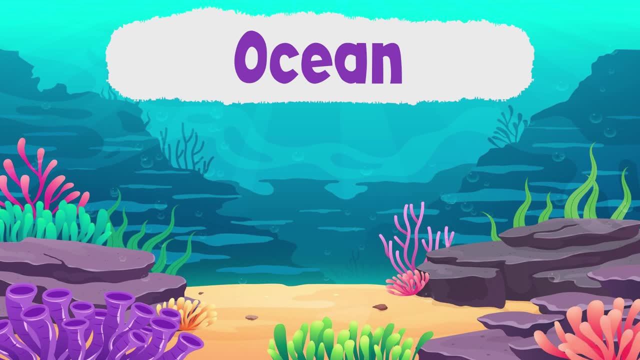 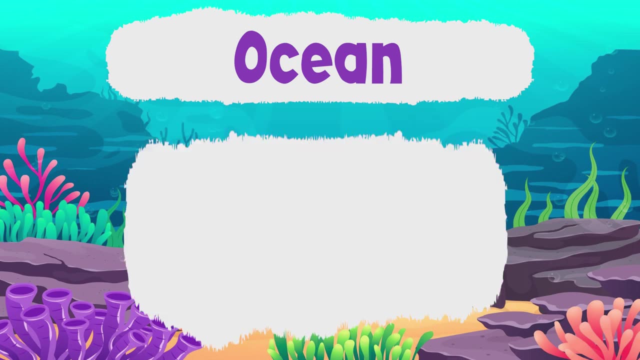 and turtles live in freshwater habitats. Ocean habitats are salty water that is very wide and deep. About 1 million kinds of animals live in the ocean. The Pacific Ocean is the largest ocean in the world. Other types of oceans are the Atlantic, the Indian. 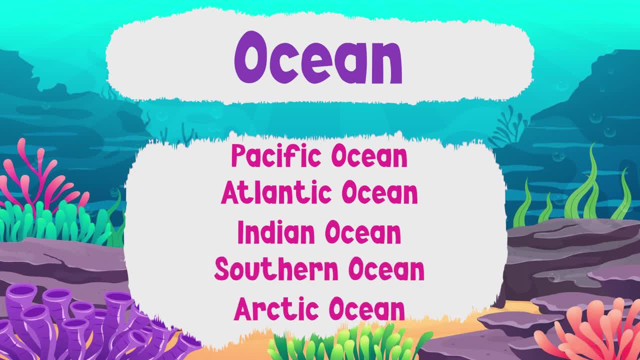 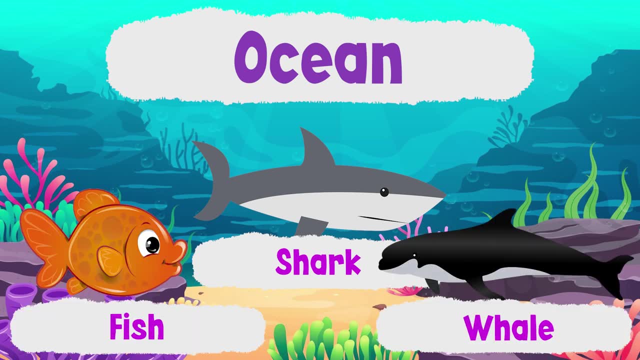 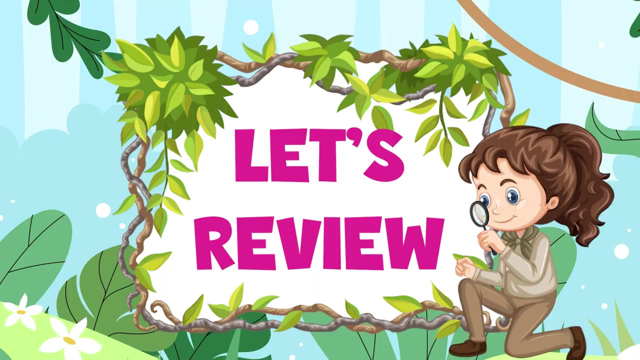 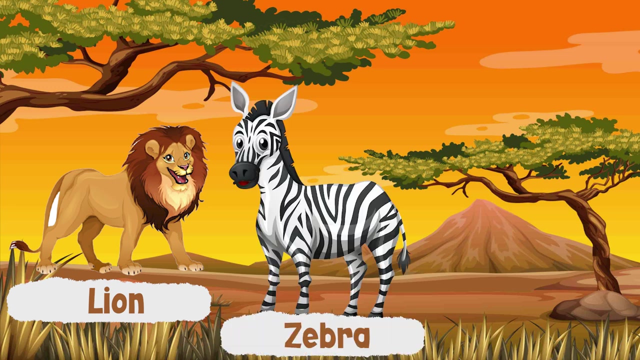 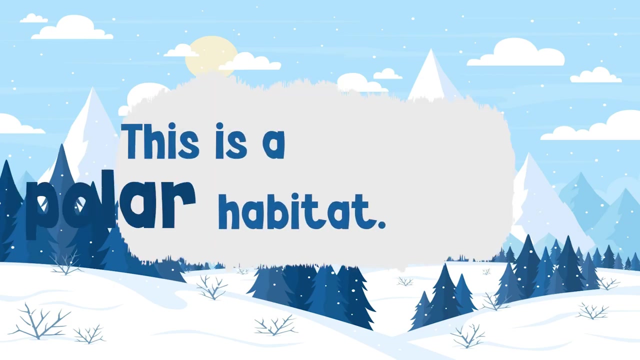 the Southern and the Arctic. Sharks, fishes and whales are some of the animals that live in the ocean. Let's review. This is a grassland. Lions, zebras and elephants live in grasslands. This is a polar habitat. 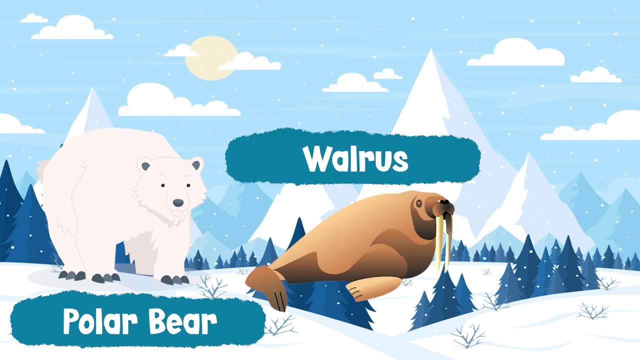 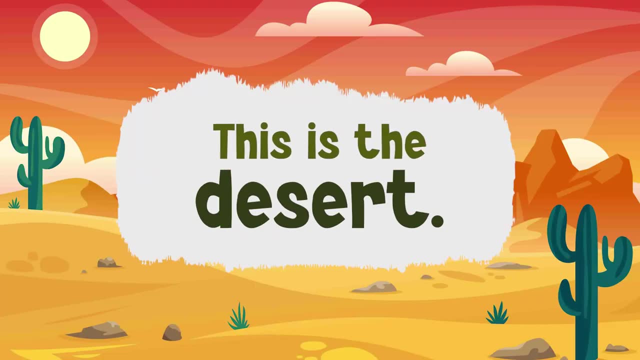 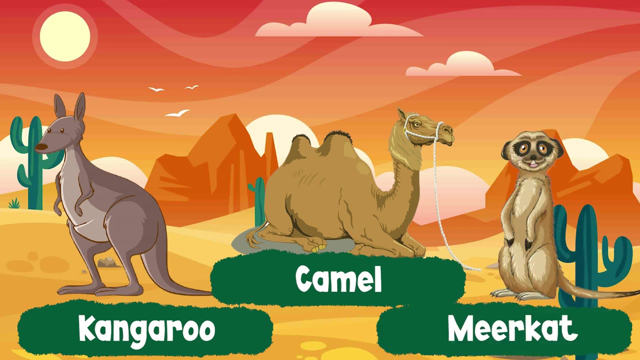 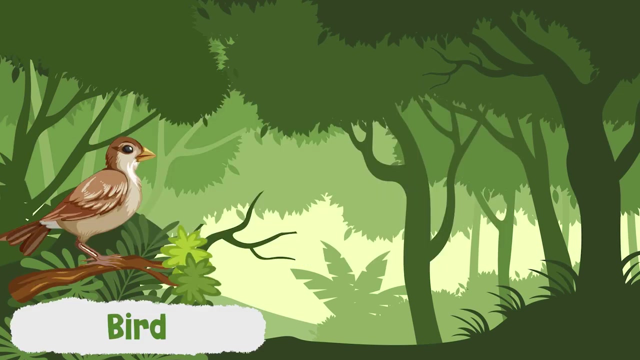 Polar bears, walruses and penguins live in polar habitats. This is the desert. Kangaroos, camels and meerkats live in the desert. This is a forest. Birds, bears and bears live in the forest. 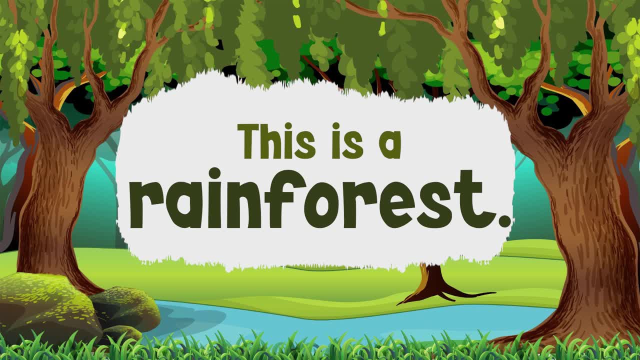 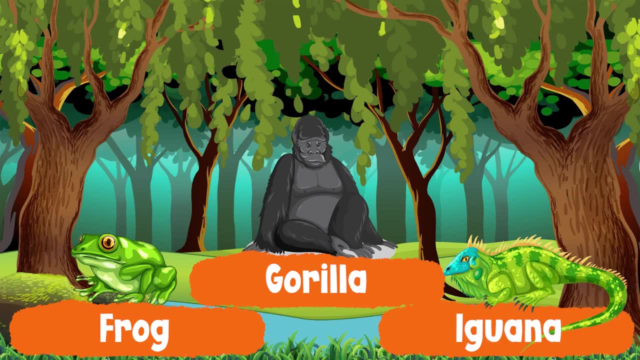 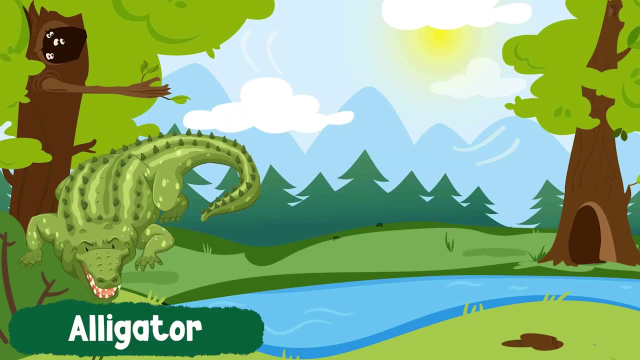 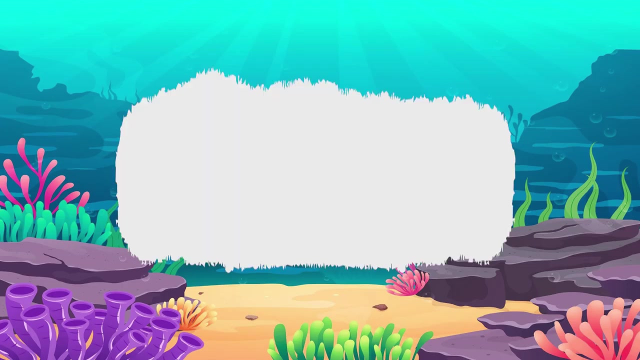 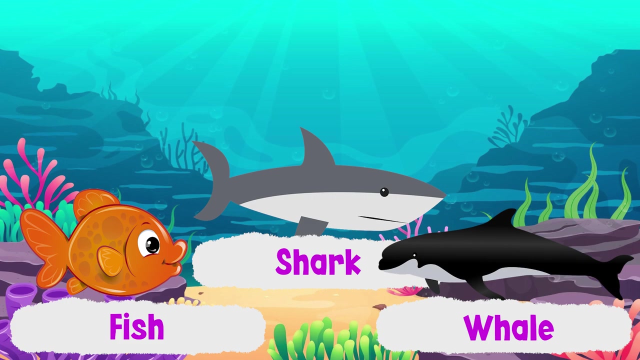 This is a rainforest. Frogs, gorillas and iguanas live in the rainforest. This is freshwater. Alligators, ducks and turtles live in freshwater habitats. This is the ocean. Sharks, fishes and whales live in the ocean. 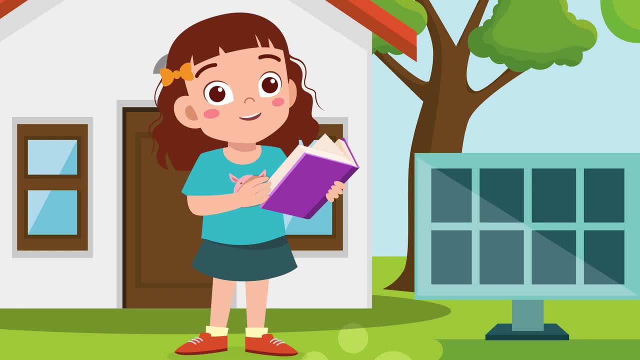 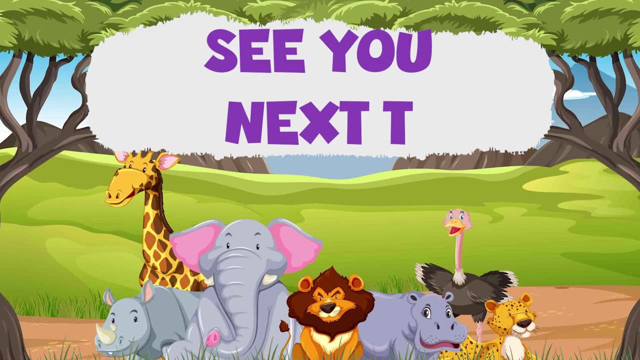 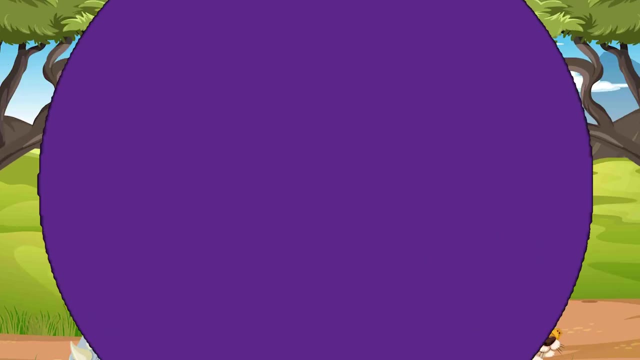 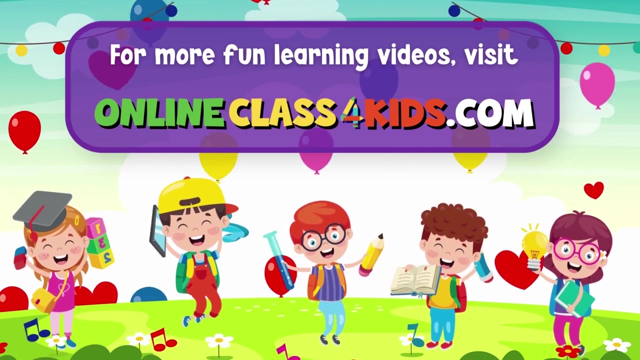 Very good, Well done. I hope you had a wonderful time learning about animal habitats. See you next time for another fun-filled learning Only here at Online Class for Kids. Visit OnlineClassForKidscom for more fun learning videos And don't forget to subscribe to our channel.